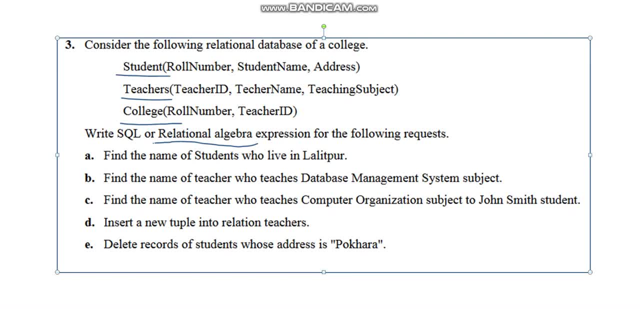 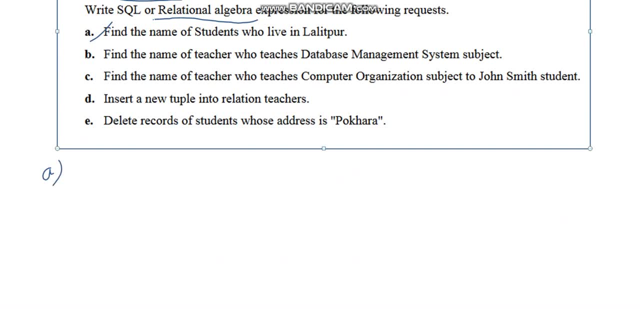 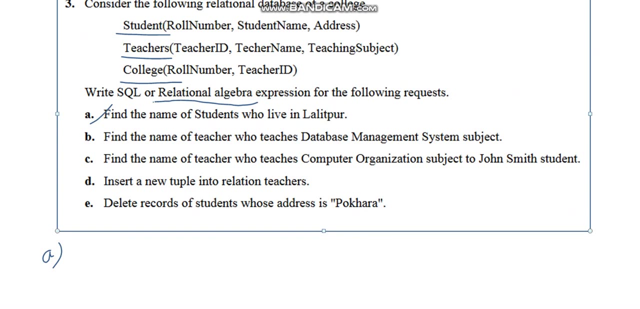 teachers in college. and let's look into the first question. let me write answer for it here, okay? so the first question says: find name of the students who live in Lalitpur. so the question is very simple: name. the attribute is name. the attribute that you have to find is name and table name is a student, because it. 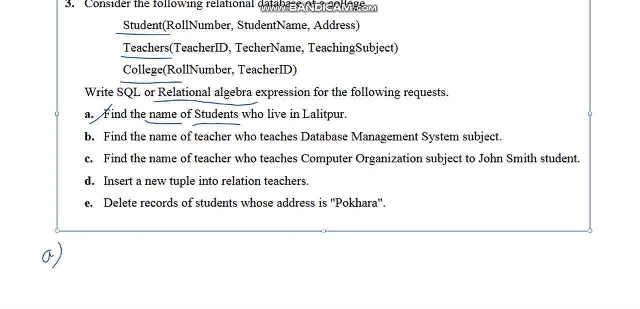 says find the name of students who live in Lalitpur. there is condition given the address is Lalitpur, so you start with PI or project operation. why? because it says only name of the attribute it. if the question was about all the attributes then you could. 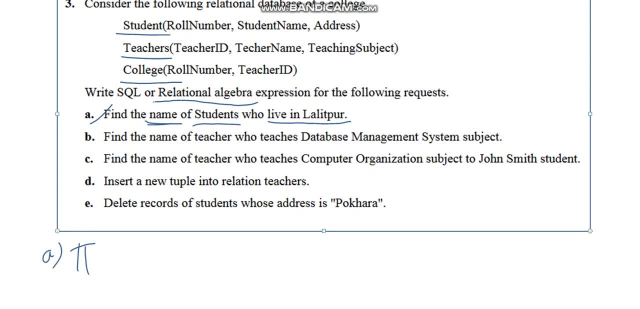 directly use the select or Sigma symbol. since they are asking only name, you have to write PI, student. excuse me, student name. okay, excuse my in writing. this is the first time I am trying with stylus. okay, so the thing, the attribute you have to find out, is: 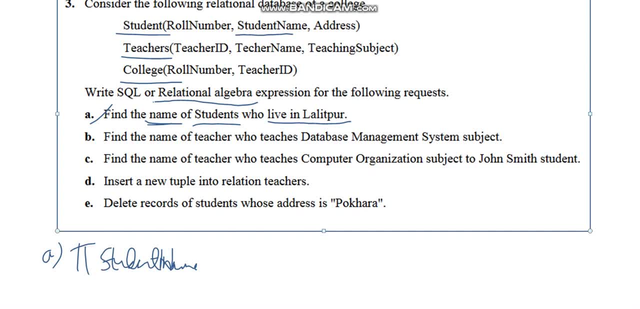 student name. this is the attribute name and from which table? from the student table and the condition. there is one condition also. condition says the predicate is address is Lalitpur, and from which table? obviously, student to not alot of difference due to to each individual path, 14 to 18 and one the 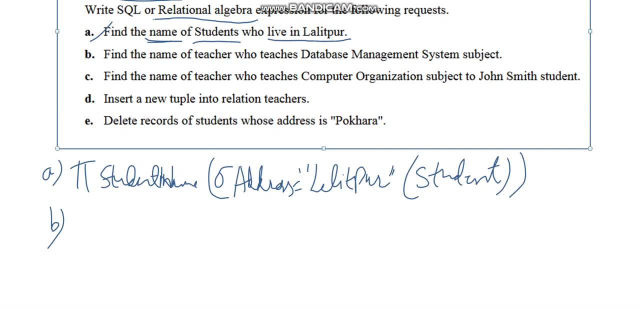 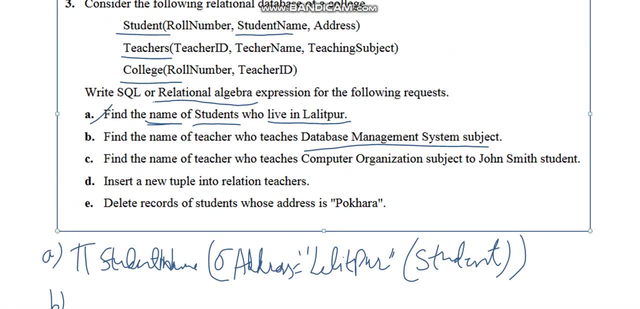 dresser is again tab to 50 WAI. let's put five red empty dot. and this is from the teacher and that is the answer you would need to have. download soccer system consists of this. question is okay. so this is the answer for machine number a. question number B says: find name of the teacher who twitches database management. 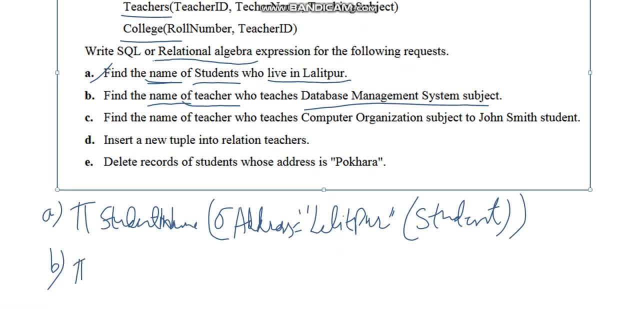 DBMS subject. so by teacher name. I'm writing the short form. you have to write the full form teacher name. yeah, from who is stable? from, obviously this teachers table. and what is the condition? the condition is: by sorry Sigma subject, sorry teaching subject: teaching. this is attribute. we are talking about teaching. 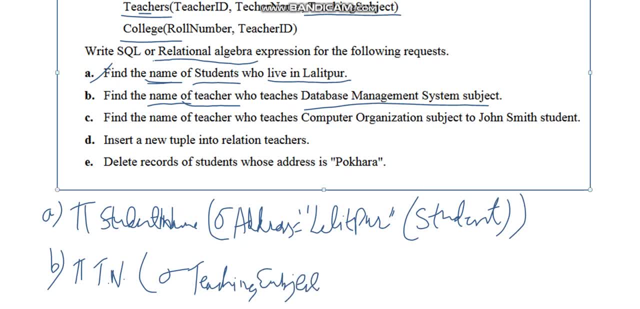 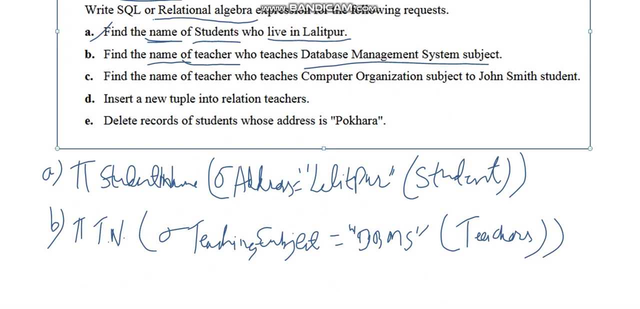 subject: subject equals to DBMS. you have to write the full form here: DBMS- data transfer. from which table from teachers tail? okay, yeah. so the question number c says question no C is hurts, not very tough, but a bit more complicated than question a and B. so here it says: find the name of the teacher who teaches computer. 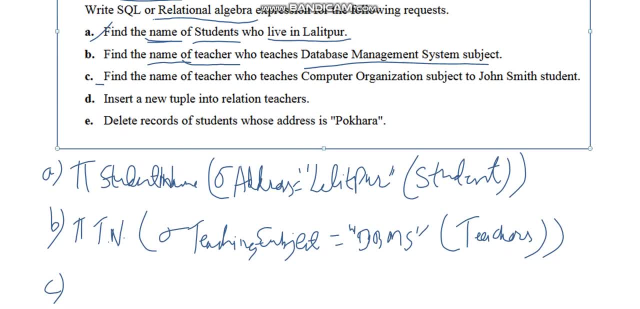 organizations. subject: tobai Smith. okay, find, find the base name of teacher who teaches computer science. subject to zon Smith. okay, find, find the base name of the teacher who teaches computer science. subject to zon smith. okay, find the. if you look into the question from here to here, if you look into this much, then this question is: 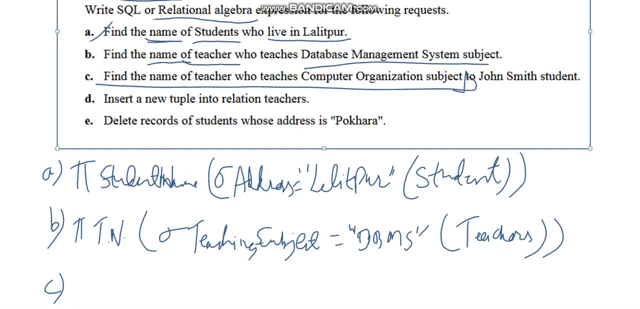 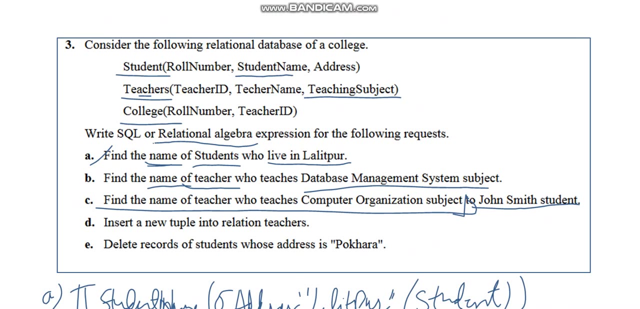 almost same as question number b. so this much is fine. but there is one more condition. condition says this particular teacher should be teaching uh to student john smith. so you have to look into conditions from these two different tables. and one more thing: if you notice, there is no common attribute between these two tables. so if there is a question which says which: 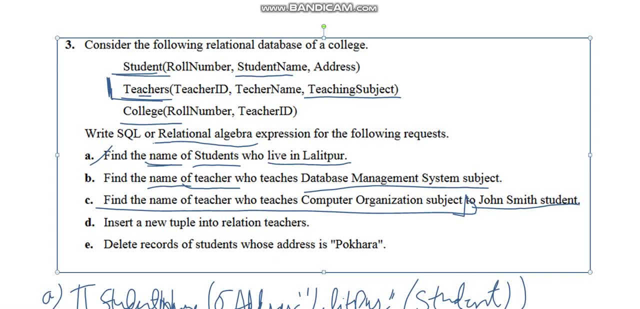 asks you to get values from two different tables, or it talks about conditions from two different tables, then obviously we are going to use something called join, natural join, and you, uh, while doing the, while performing the natural join, you have to make sure there is a common attribute. if you look into only these two tables, there is no common attribute, but if you include, 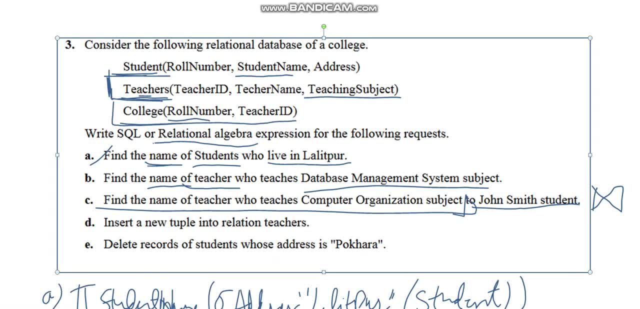 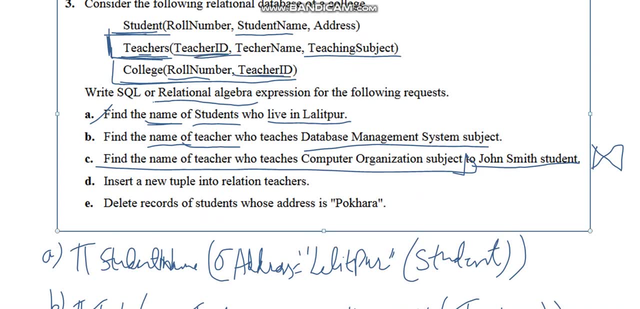 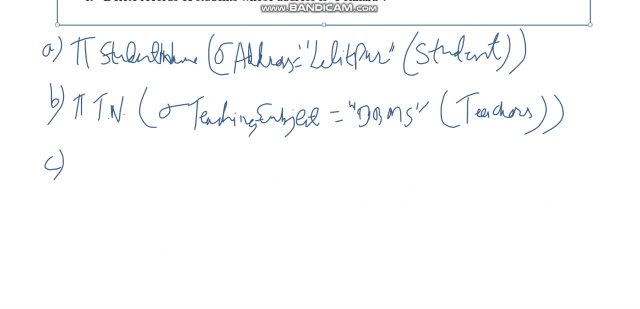 this table also, then these three tables are going to have common attributes: teachers and college share this common attribute: teacher id and student and college share role number. okay, so, uh, i'm just writing the right most part of the expression, that is: student join college join teachers. okay, this is. 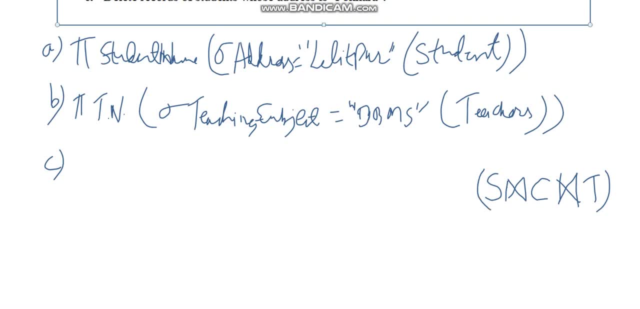 the right most part. from which table? uh, you have to find the, find the values from the table joined, okay, join table, which is a join of student, college and teachers. uh, you have to write the full form just to say the space and, due to this stylus issue, i'm writing the shortcut. okay, so this is the right most part. 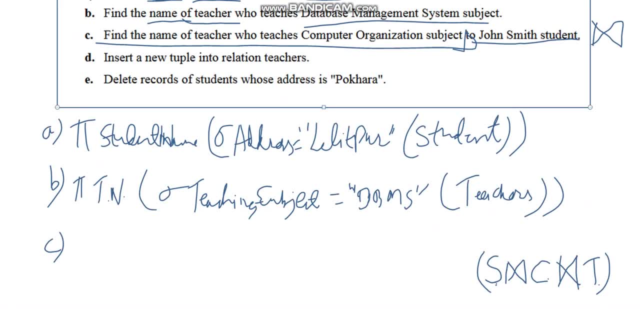 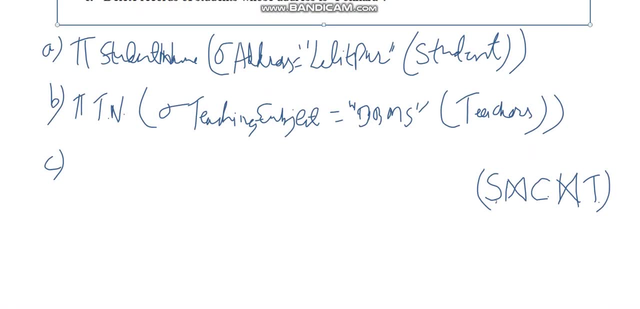 and, and there is a condition also, and what you have to find out is name of the teacher, so you can just start with writing by teacher name. okay, teacher name, uh. and the condition is the teaching's subject should be computer organization. and- and there is one more condition- the student name, what? 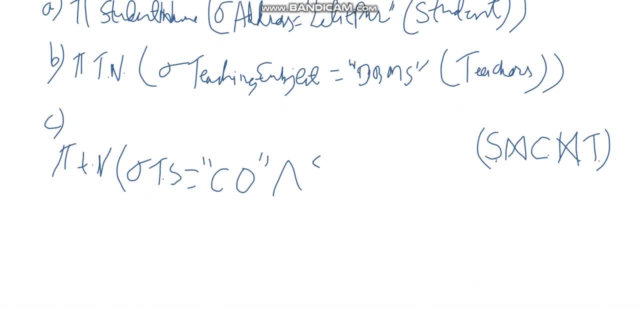 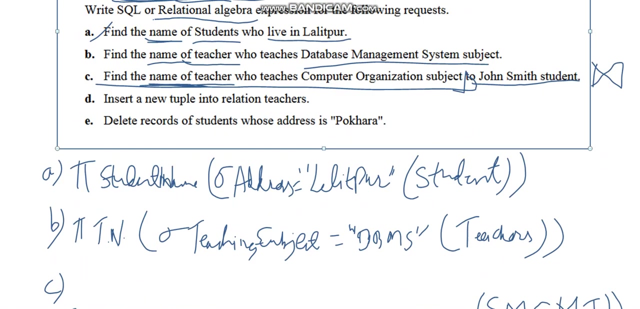 is the yeah student name. student name should be john smith. you just have to write the full forms. okay, i'm just trying to save the space. okay, yeah, and another closing bracket here. this is the relational algebra expression for this. and question number d says: insert a new tuple into relation teachers. so while inserting, you use, you make use of. 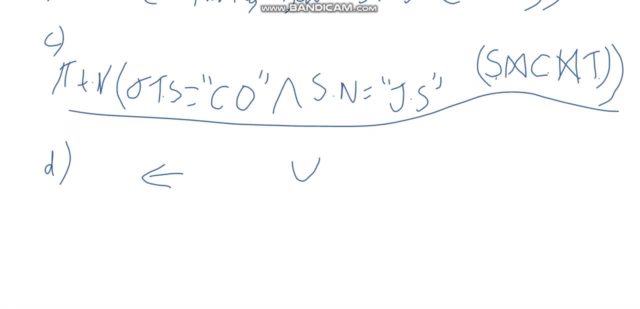 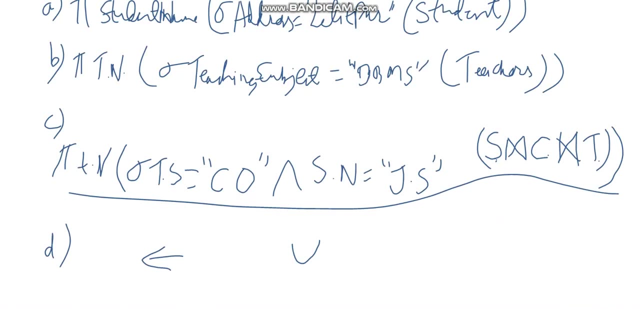 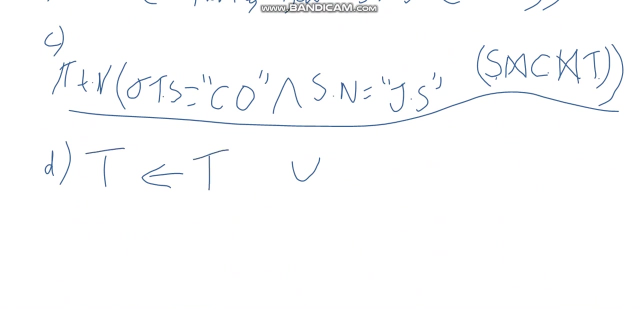 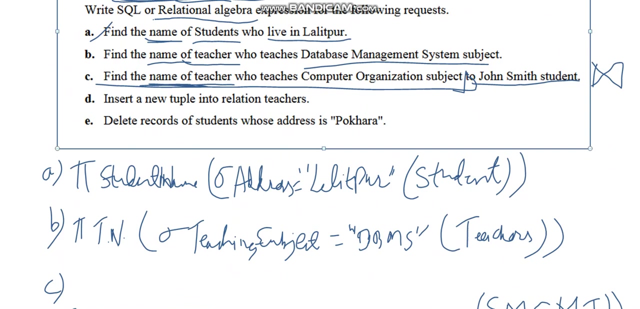 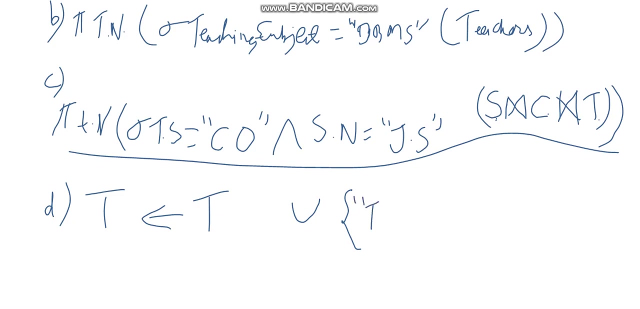 assignment operator and union operator right for insert operations. and what is the name of the table? table name is teachers. okay, so teachers equals to uh, teachers union, union of a set of new values. just write some random values. make sure the values correspond to attributes. but you can write anything here: teachers, teacher id, teacher name and teaching subject, teacher id. 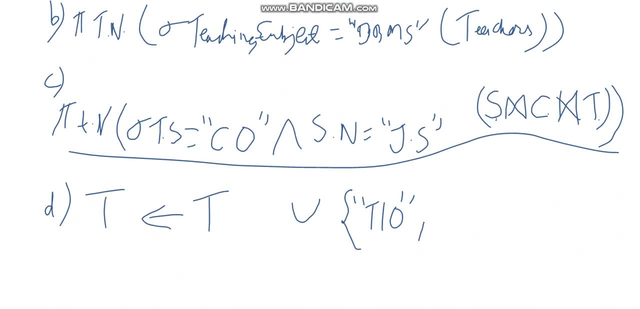 be anything. i'm just writing t10 and teacher's name can be anything, any name, and the subject he teaches, for example, java. okay, this statement, just write the full form: teachers here, teachers here. and this statement or this relational algebra expression will insert a new tuple into teachers table. okay, and yeah. question number e: 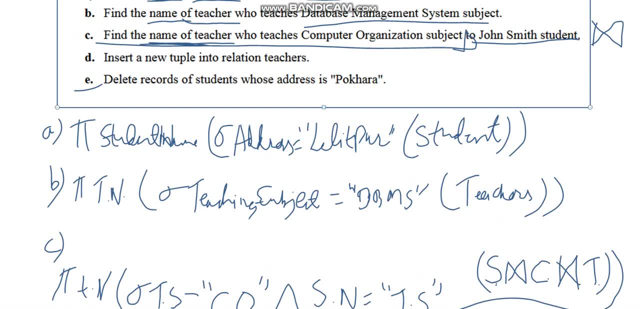 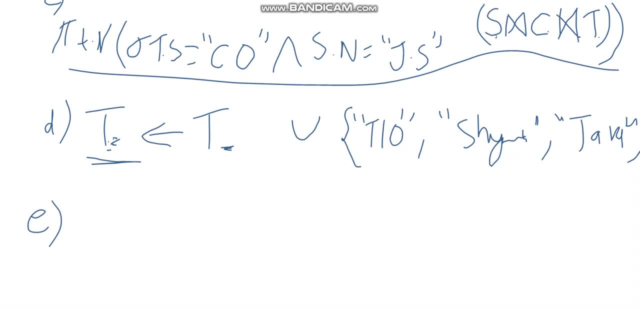 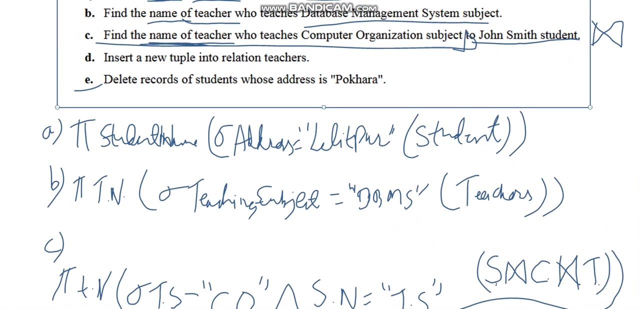 delete records of students whose address is pokhara. so the question number e says: delete records from students from his table. so a student is assigned a student minus instead of union. we are using minus here because we are deleting a tuple now, and which tuples were whose address is pokhara. 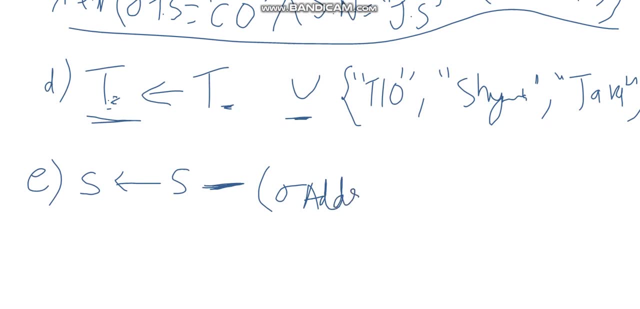 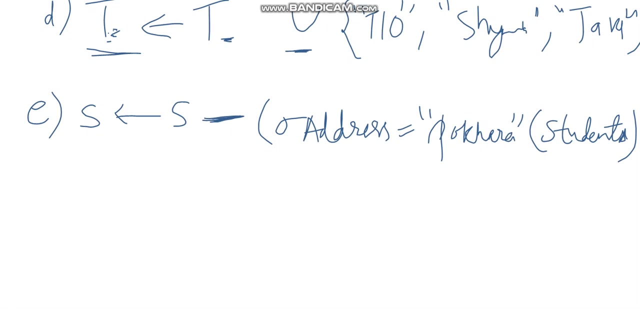 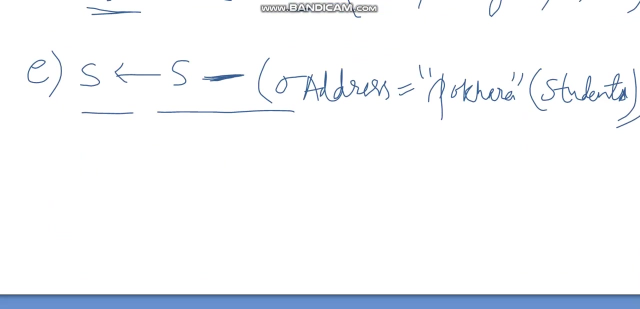 that means sigma address equals to pokhara. okay, from his table students, or is it a student? okay, only student. no s here, only student. and yeah, this minus this, this will give you the. this will, uh, remove tuples from the table students whose address is pokhara. okay, thank. 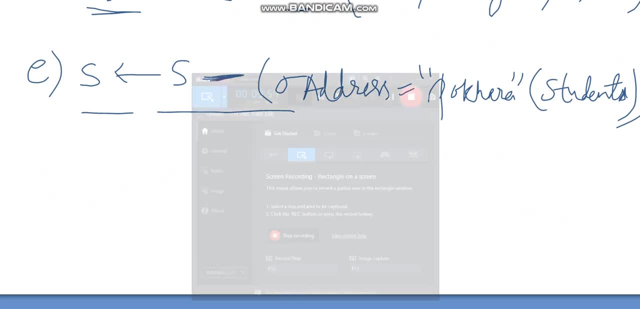 you. i hope it helps.